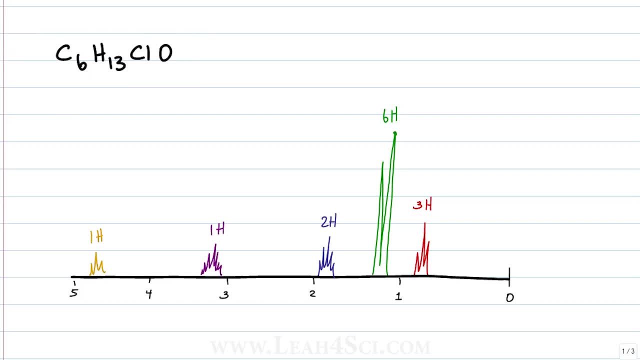 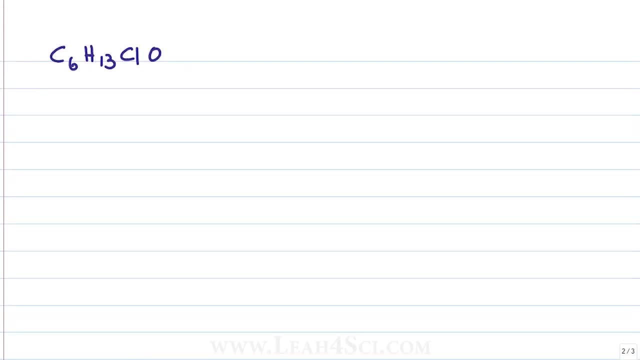 do when you're given the molecular formula is to figure out your index of hydrogen deficiency so that you know if to consider any pi bonds or rings. To do that we'll use the equation CNH2N plus 2, which I teach in the index of hydrogen deficiency. video linked below: N. 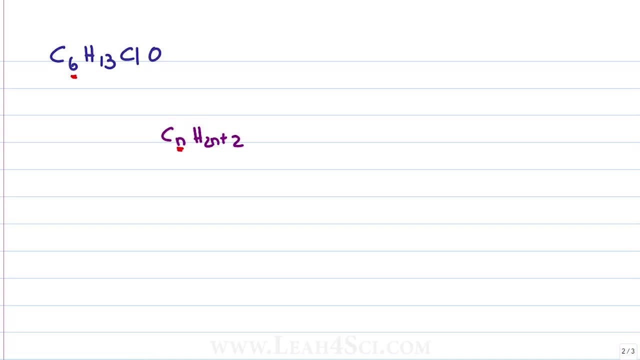 represents the number of carbon atoms. in this case we have 6.. So if we set it up as 2N plus 2 to solve for hydrogen, we have 2 times 6 plus 2, where 2 times 6 is 12 plus. 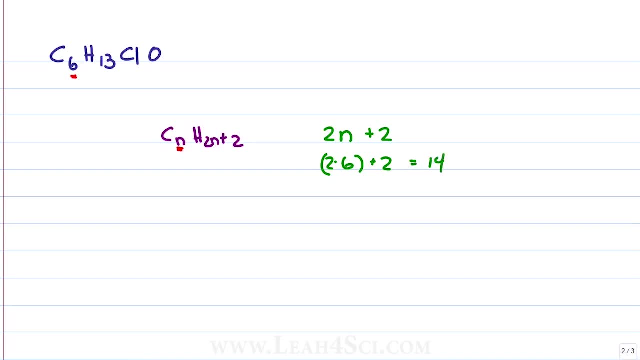 2 is equal to 14.. If we have the maximum number of hydrogens, we know we have a fully saturated molecule with no pi bonds and no rings. But in this case we only have 13 hydrogens. So what does that mean? It has to be an even number. Don't forget that. halogens, because 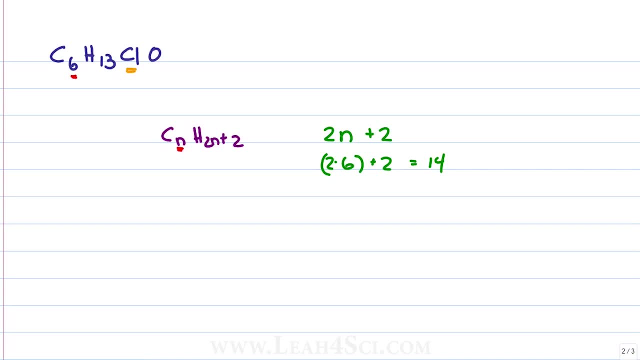 of how they bind to carbon count, just like hydrogen. So if we add up 13 hydrogen plus one hydrogen like halogen, we actually have 14.. With that we get 13.. So we have 13 hydrogen plus one hydrogen like hydrogen, which is equal to 14. The number of hydrogen is equal to. 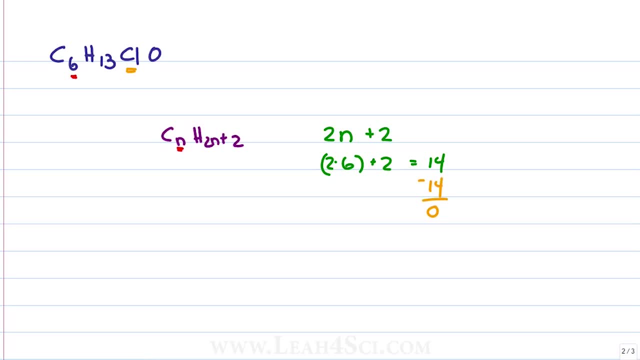 14,. 14 minus 14 is 0. that means we have no pi bonds and no rings on this molecule. This helps us when we look at the structure, because we know we don't have to consider anything crazy. This also helps us with the oxygen, because it immediately rules out anything with a carbonyl. 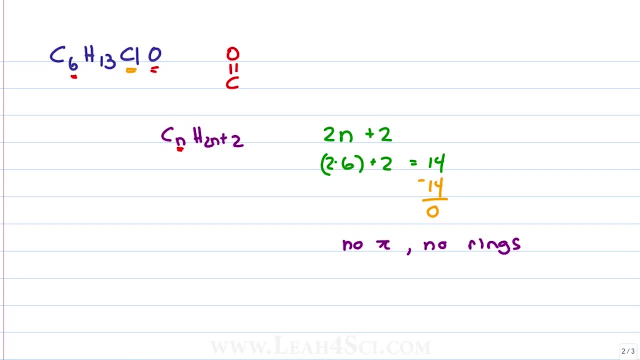 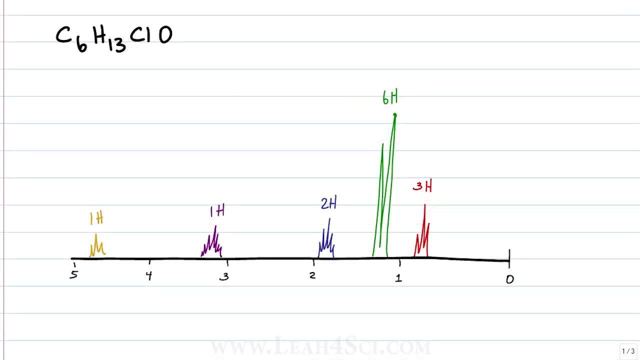 Remember, a carbonyl is a carbon double bound to oxygen, which would require an index of hydrogen deficiency. Now that we have an idea for the molecule, let's take a look at the graph. I'm going to break this down and solve it the way I teach in my beginner NMR videos. 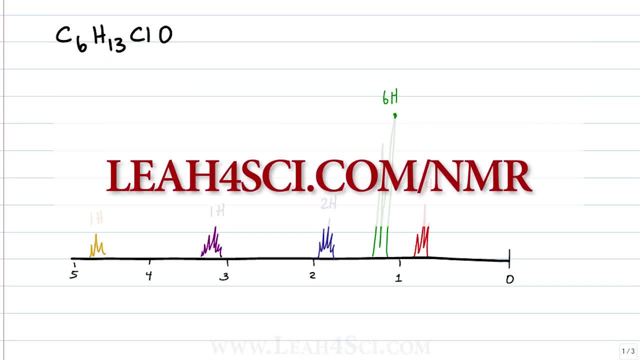 which you can find linked below or by going to my website, leah4scicom. slash NMR. I consider the right side of the graph anything near 0, the boring region. This means that the carbons and hydrogens on the right are further away from the exciting. 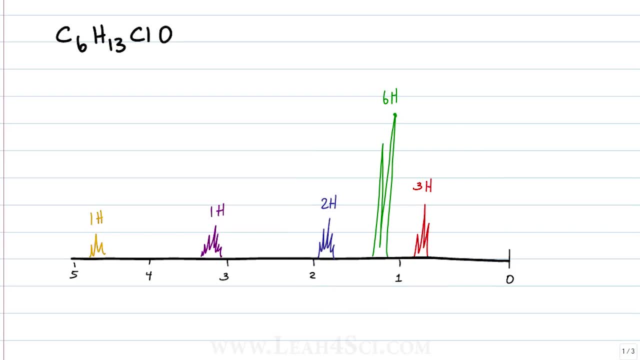 groups like halogen and oxygen in our case, And the left is the hydrogen And the right is the exciting group. That means these two are likely sitting close to the oxygen and the chlorine. I drew the peaks in different colors so that we can refer to them by color and have a very 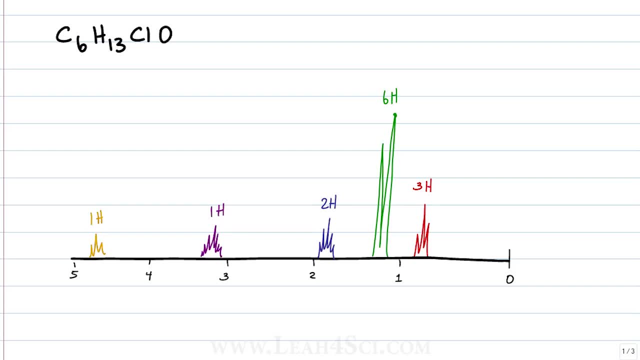 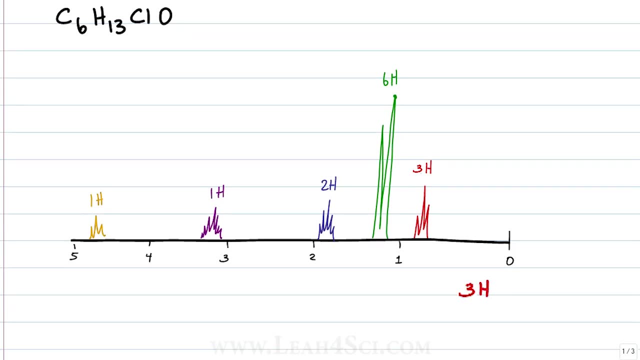 clear idea of what we're looking at. Let's analyze them, starting from the right, where we have three hydrogens. So three hydrogens is going to be the CH3 with the peak of a triplet. How do we know it's a triplet? 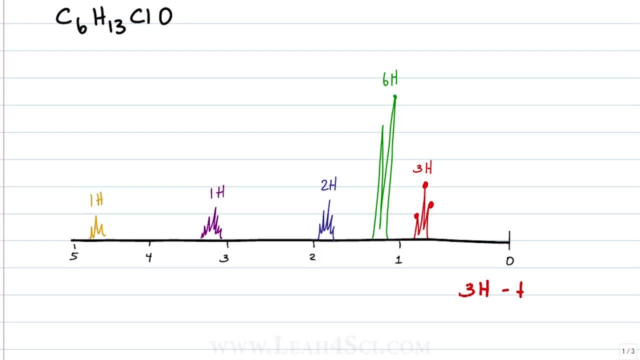 We can count three distinct tops right, So this is three. Three points for a triplet. We'll use N minus 1 to find the number of neighbors. So three points minus 1 tells us that we have two neighbors nearby. This right here is a CH3 group. 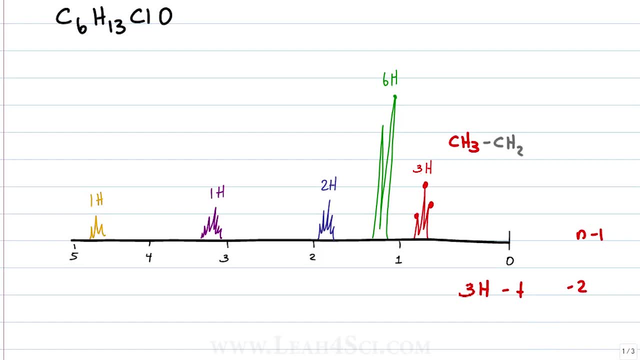 I'll draw the ghost atoms in gray so we know not to count them as part of our molecules. But if we can match up a ghost to another piece, we know that we have a puzzle coming together. For the green peak we have six hydrogens. 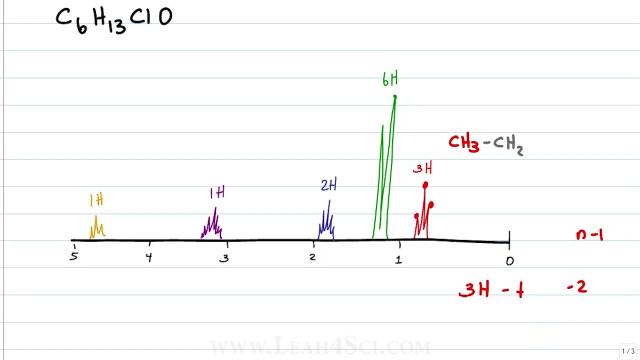 This has to be two carbons, because one carbon can have a maximum of four bonds, but six hydrogens have to be sitting on two equivalent carbons, meaning there's some sort of symmetry there. And having a doublet meaning- two points- tells us that we have only one neighbor. 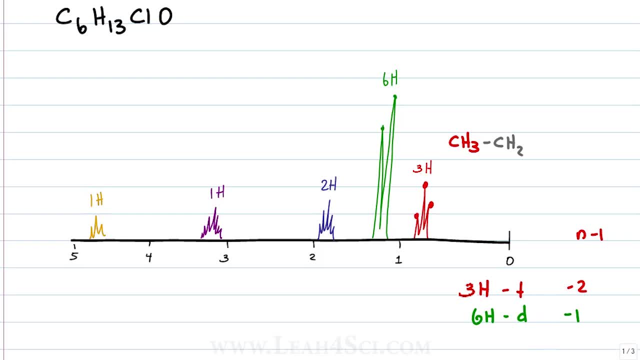 Two minus one is equal to one. That means there's one neighbor for these two different CH3 groups, which means we have a CH3, another CH3.. Six hydrogens have to be sitting on two equivalent carbons. That means we have a triplet. 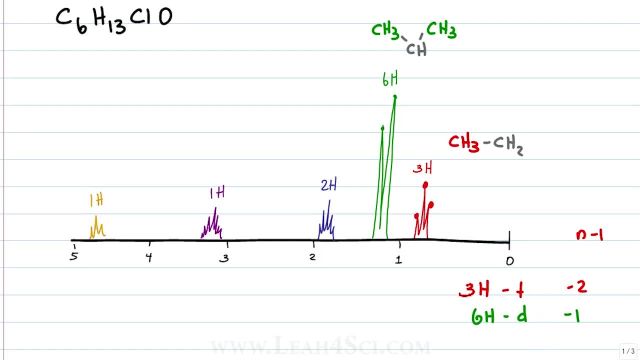 We have a triplet sitting next to a carbon that has one hydrogen splitting them both. I wanna jump over to the purple peak real quick, because this is a pattern that you have to learn to recognize Anytime. you have a six hydrogen doublet and a one hydrogen multiplet, which is this mass. 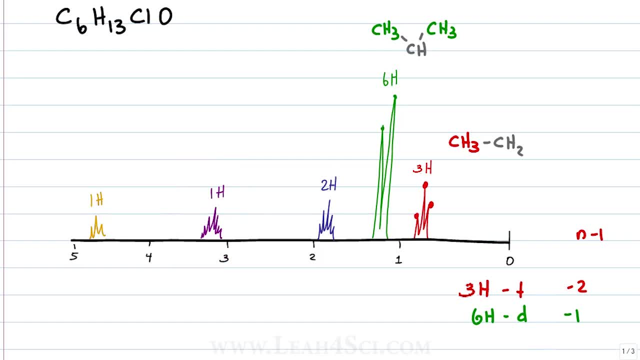 over here. you should recognize this as an isopropyl group. The purple group is one hydrogen. specifically, we have a septet, meaning we have seven points, but you'll often see this just called multiplet, because anything over five or six becomes. 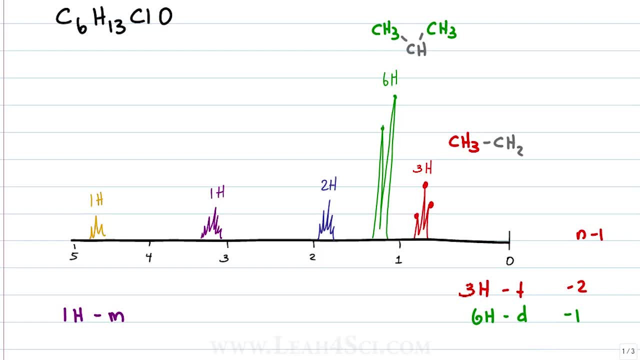 too messy. So we recognize: oh yeah, it's got a whole lot of neighbors. In this case, septet is seven. seven minus one is six neighbors. well, what other six neighbors would it be, if not for our six hydrogen 2CH3 groups? 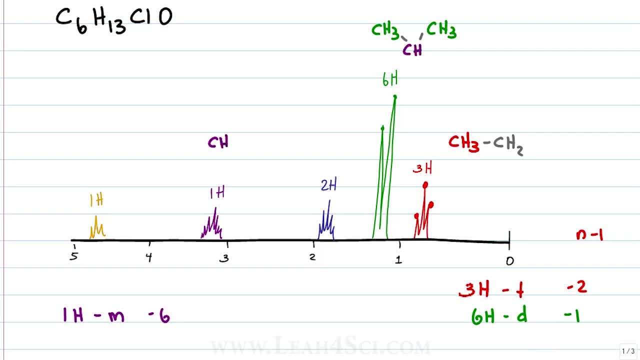 So let's go ahead and put that right in here. no more ghost CH, that right, there is an isopropyl group, So we have one piece of the molecule. Let's go back to the blue two hydrogen group. We have two hydrogens with a quintet. notice, we have five points. a quintet is five minus. 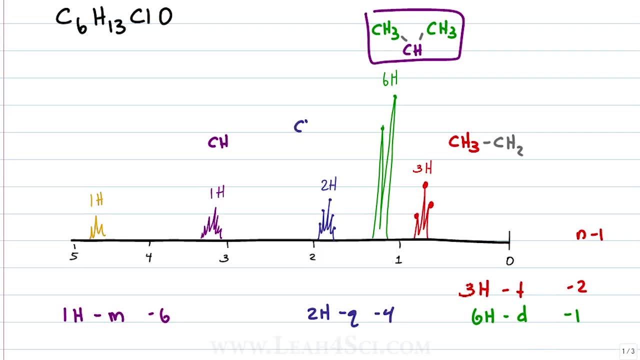 one tells us that we have four neighbors, and the four neighbors could be one of two things: I can have a CH2 group on either side which adds up to four, or I can have a CH3 on one side and a CH on the other. 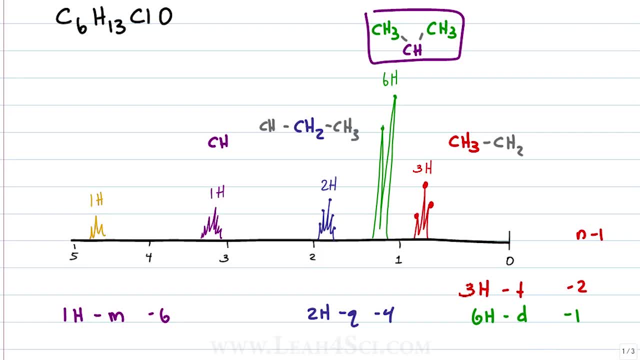 In this case we know it has to be a CH3 on one side and a CH on the other, because this is the only peak on this graph that has two hydrogens. We have no other CH2s visible because nothing else has two hydrogens. 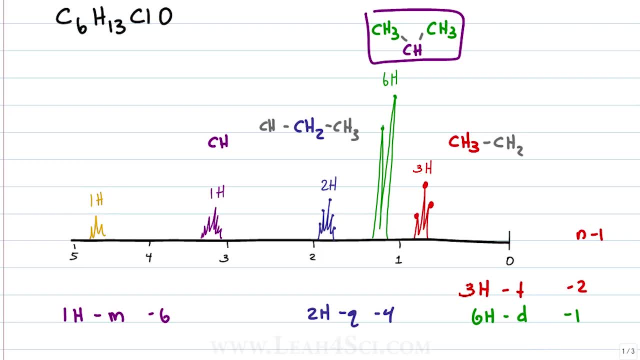 Last but not least, the brown group on the left- is one hydrogen In a triplet. we've already said that a triplet is three minus one for two neighbors, and that means this CH has a CH2 nearby. Now notice, we haven't even considered the oxygen and the chlorine yet, and the reason 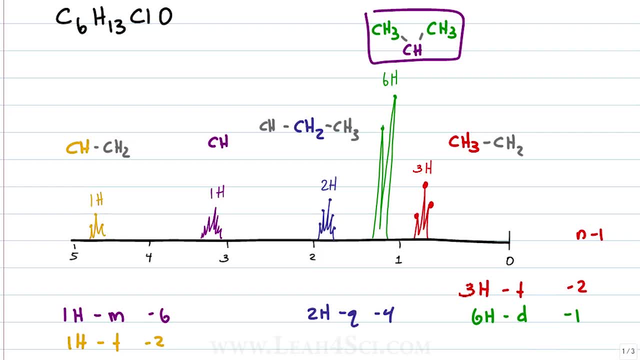 for that is intentional. A lot of students will try to match everything up at the same time, but if you let the carbons themselves match up like puzzle pieces that click, then typically the rest of the groups will fall into place and if not, you wanna take extra steps to figure out where they. 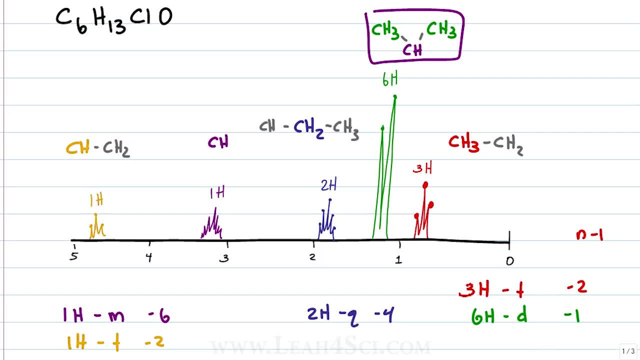 go. but why waste the energy if you don't have to? Before we start putting everything together, let's make sure we accounted for all six carbon atoms. Sometimes you'll have, say, a carbonyl that doesn't have any hydrogen, and you have to. 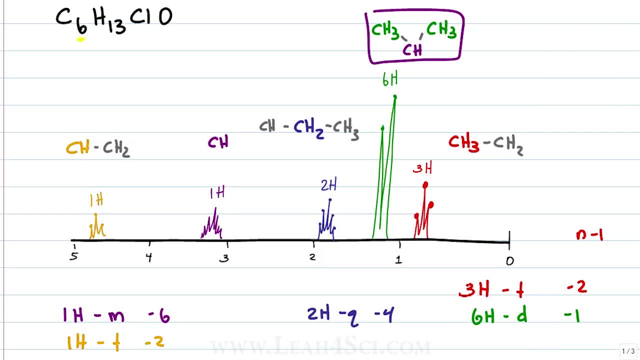 remember to create another puzzle piece on the side to take into consideration. So what do we have? One carbon, two carbons, so that's three. another carbon is four, another is five, another is six. all of the carbons are accounted for. 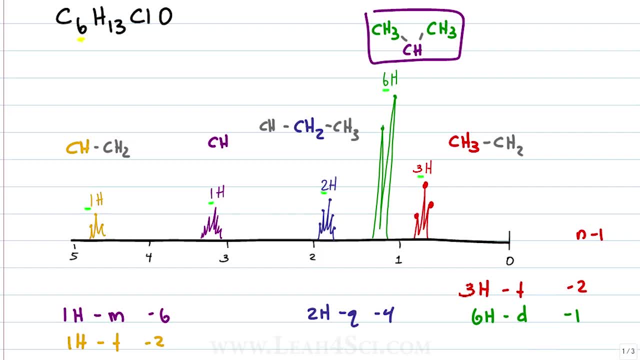 Now look at our ghost groups. For the ghost groups. are there any ghost groups that match up A group that we have? For example, we know we have a CH3, this is the only CH3. I don't even need to look at the shift to see if they match up. I have no other option. 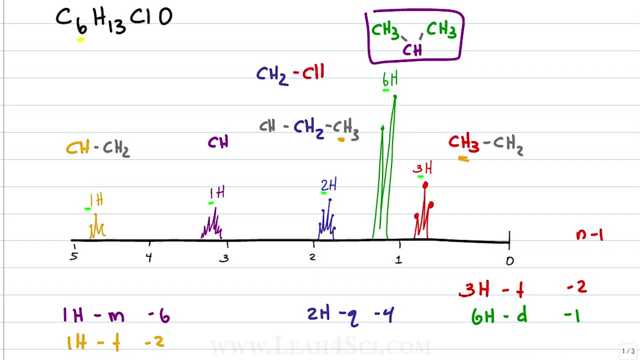 So that tells me that the blue CH2 has a red CH3 on the side. We accounted for this- let's cross it out: same here- And we also accounted for this in the isopropyl group. The only thing that's missing is the brown CH. well, we know that we have to have another. 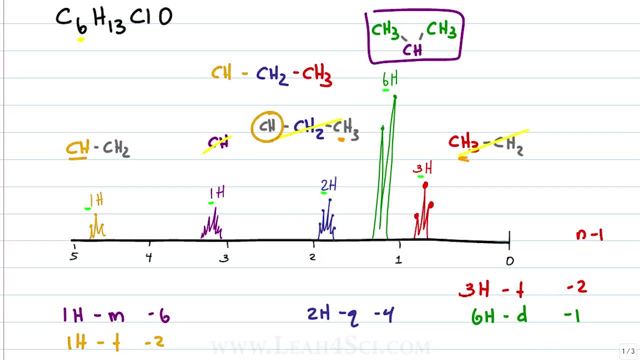 CH on the other side of the blue group, so let's go ahead and put that CH right there And that's it. we practically have the entire molecule put together. where we have two portions of the molecule, One portion is an isopropyl group, the other one is a regular propyl group. 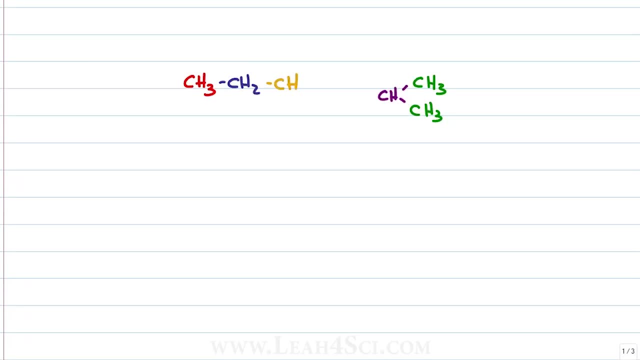 Now what? This is where it gets exciting. We have two pieces. we want to see how they connect. we also know we're still missing an oxygen and a chlorine. If you count up the bonds that are here, you'll recognize that the brown CH is the one that's. 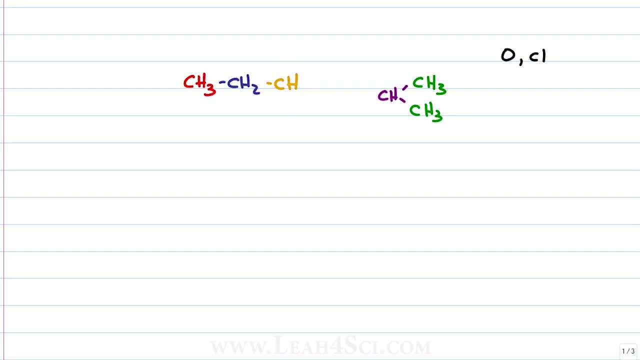 missing. So what do we have? We have two pieces. The purple CH can have two more bonds, because it needs to have a total of four, And the purple CH already having three bonds- two to the methyl groups and one to the purple hydrogen- can have just one more bond. 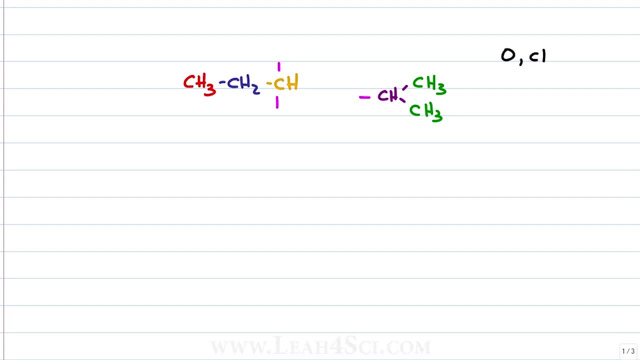 I challenge you to figure out the rest of this without even looking at the graph. We know we have to have an oxygen somewhere. well, this one's got to have the oxygen because it's got two things, so it's actually got to have the oxygen and the chlorine. 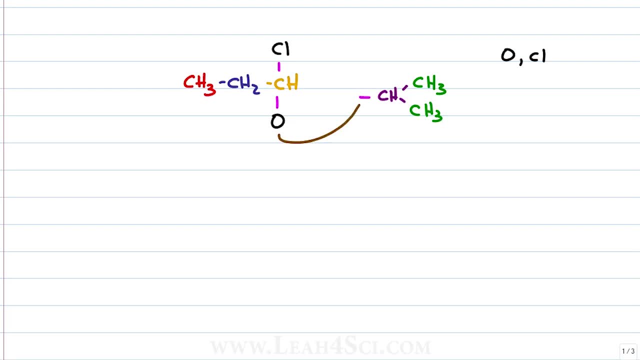 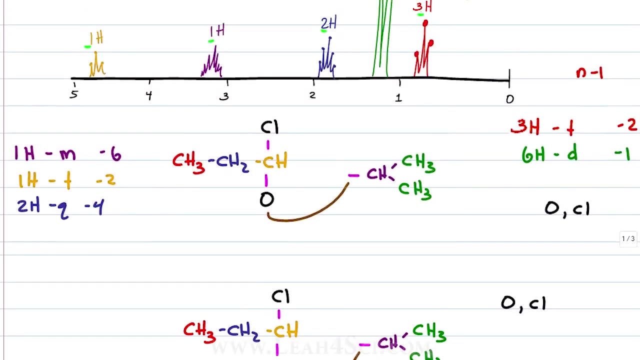 And the only way to make this one molecule is to attach these two together. So, without even looking at where the shifts are happening, we figured out the molecule. but I do want to take you back to the graph to prove it. How did we know that the oxygen was an ether rather than an alcohol? 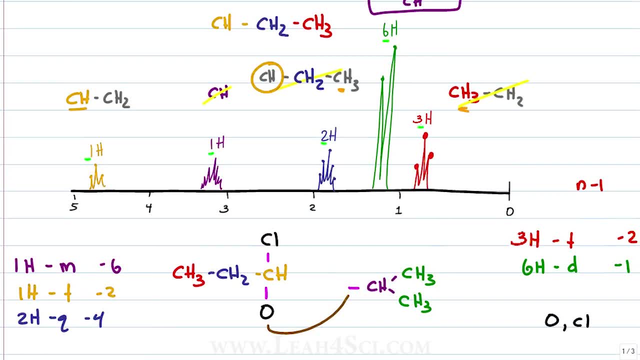 Simple. An alcohol is an OH and that hydrogen would show up as a broad short singlet on the graph. If you look at the graph, we don't have any singlets. that tells us we don't have any alcohols. We've already ruled out the possibility of a carbonyl when we found the index of hydrogen. 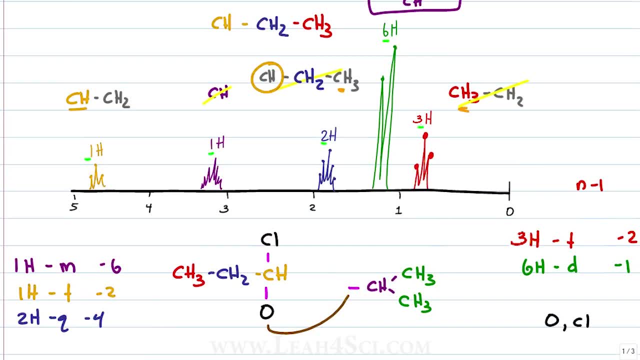 deficiency to be zero, leaving us an ether where an oxygen is bound to two other carbon atoms as our only option. We know that halogens are considered exciting. they're highly electronegative and they tend to pull the nearby carbons and hydrogens towards the four range. a little bit higher, a little. 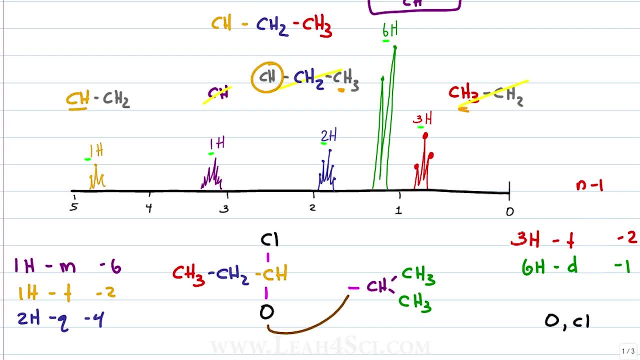 bit lower, depending on what else is going on and which halogen we have. We said that The brown CH is holding the chlorine. well, guess what? The brown CH is the highest shifted group. it is the most exciting, and doesn't that make. 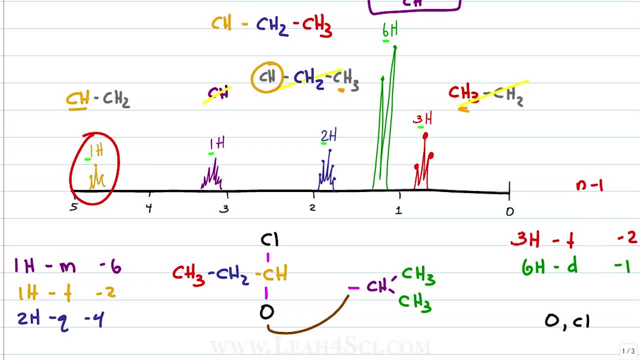 sense, given that it's next to both chlorine and oxygen and the purple CH is the second most exciting group. it's the second highest shifted- and doesn't that make sense if it's directly attached to the oxygen but not also holding a chlorine? Okay? 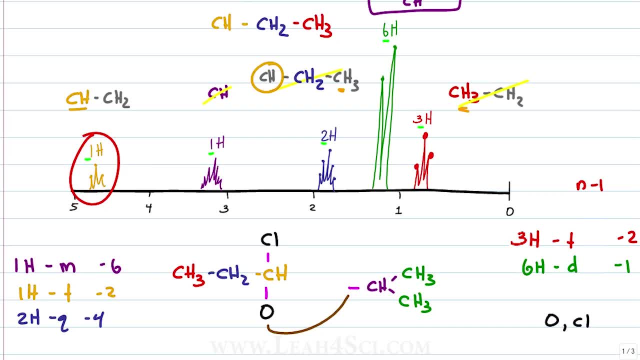 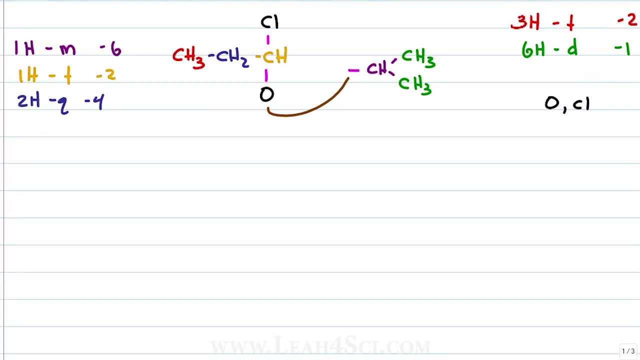 So now we've matched everything up and we have all our puzzle pieces together. The final step is to draw this into some sort of a coherent molecule, because right now it looks like a mess. I'll draw it out with all the atoms first. then we'll do an aligned structure. 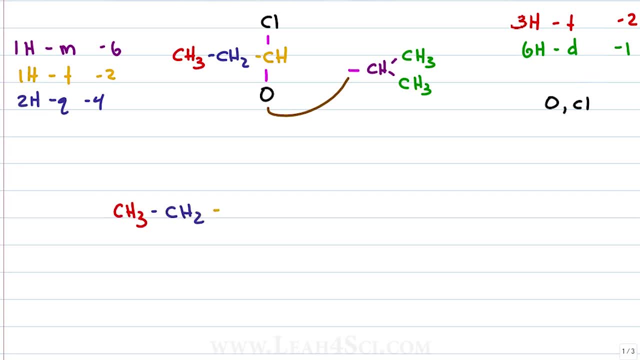 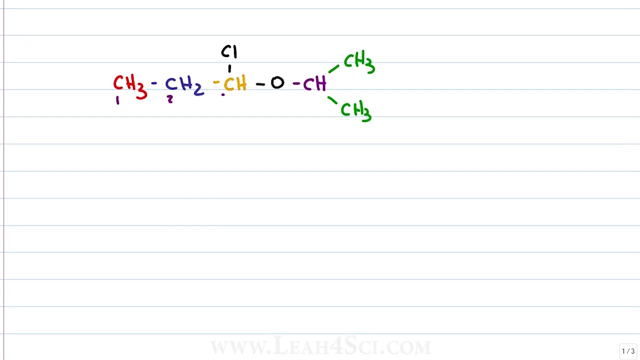 So we have a CH3 bound to a CH2 bound to a CH that is also holding a chlorine. then we have an oxygen bound to the purple CH bound to two green CH3 groups, An aligned structure that gives us one, two, three carbons, where the third carbon is holding. 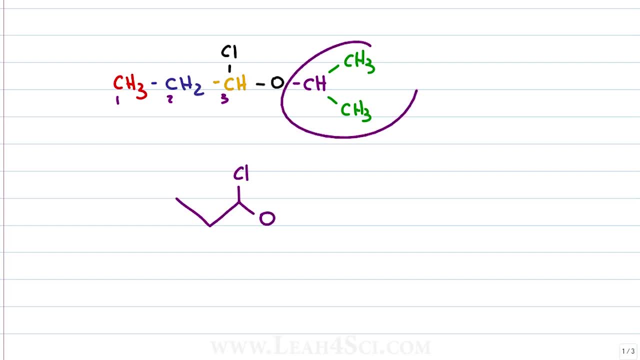 a chlorine and bound to an oxygen, and attached to that we have an isopropyl group. And there you have it. there's our molecule that came together by analyzing the pieces. If you found this video helpful, first give this video a thumbs up and make sure you subscribe. 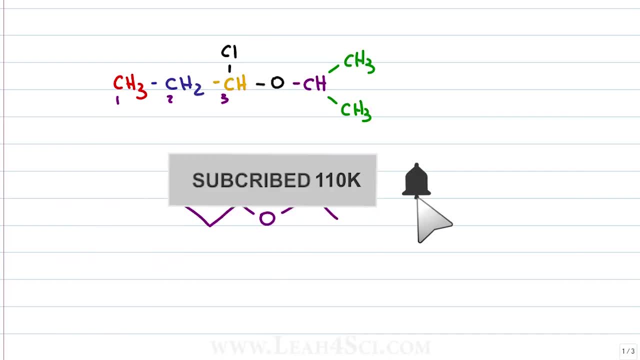 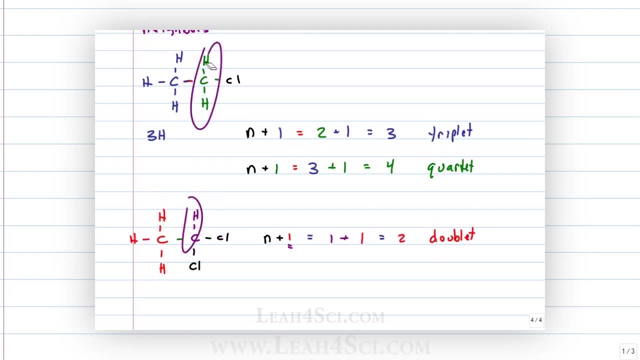 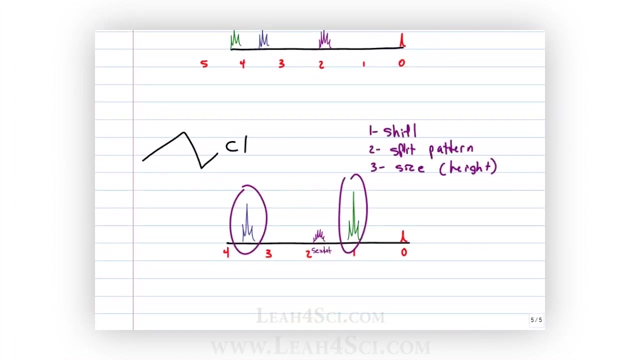 to my channel so that you don't miss out on any of the new videos. to follow this semester, I work through even more complex spectroscopy problems. I'll see you next time. Bye, bye.